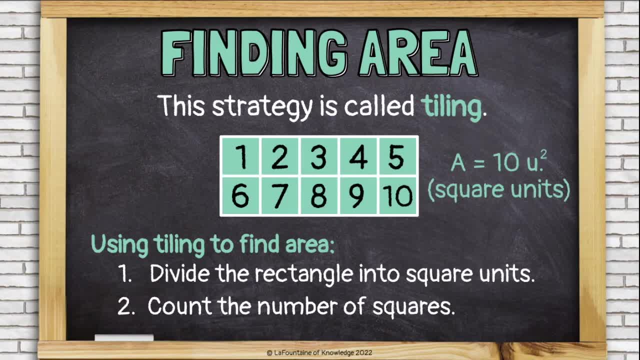 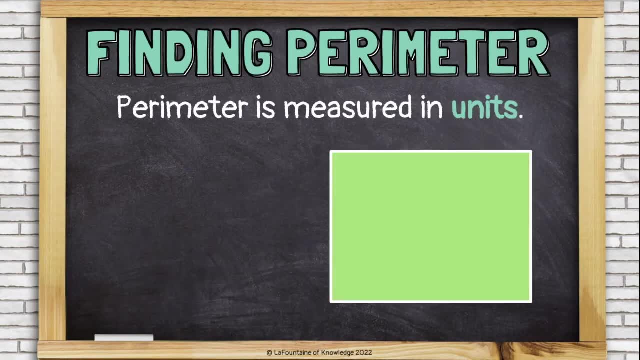 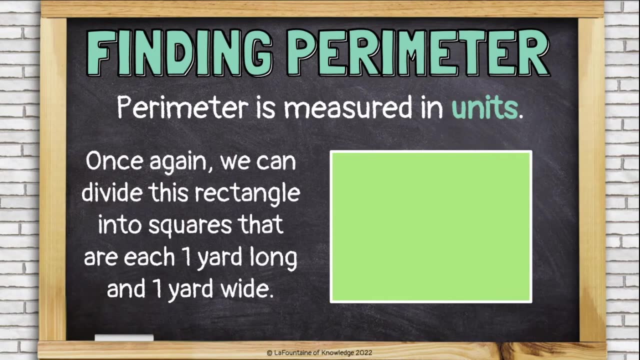 square units. now those units might be feet or meters or miles or inches, but we haven't given it a specific unit, so we're just saying units here. to be general, perimeter is measured in units, not square units. so once again we can divide this rectangle into squares. 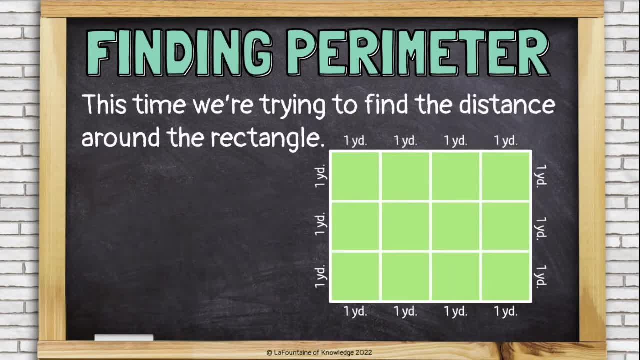 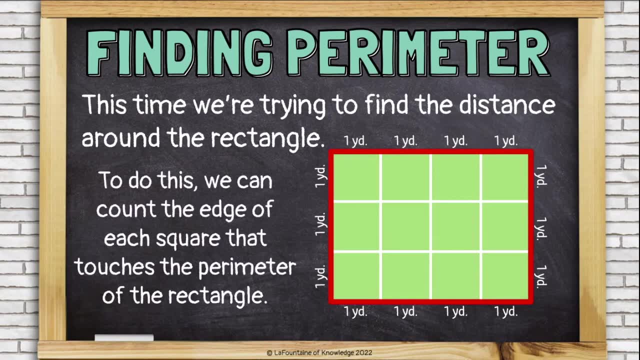 this time they're each one yard long and one yard wide. we're trying to find the distance around the rectangle. to do this, we can count the edge of each square that touches the perimeter of the rectangle like this: one, two, three, four, five, six, seven, eight, nine, ten, eleven, twelve, thirteen, fourteen. 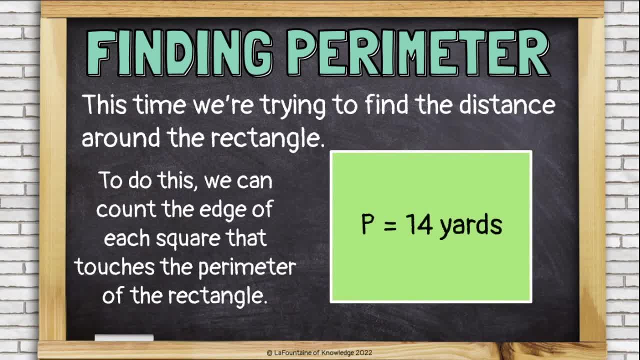 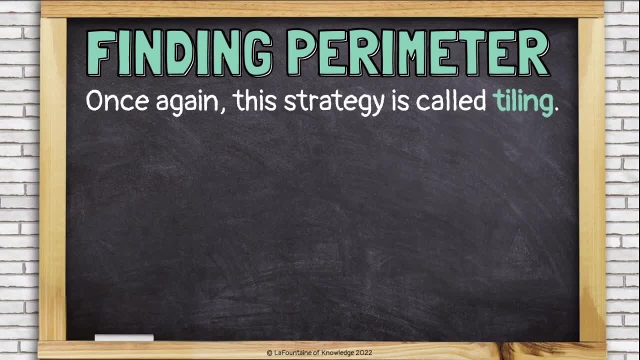 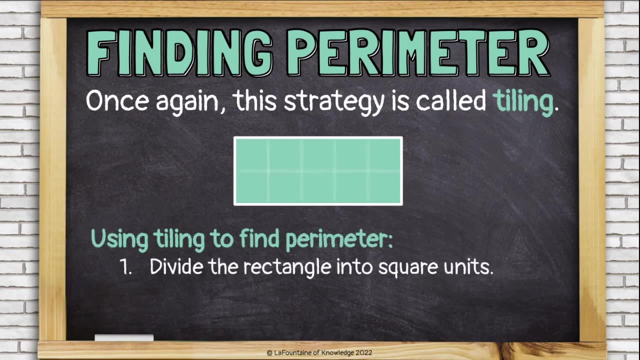 this rectangle has a perimeter of 14 yards. once again, this strategy of dividing it up into squares is called tiling. let's use tiling to find the perimeter of this rectangle. divide the rectangle into square units. count the edges of each square that touches the perimeter of the rectangle. one. 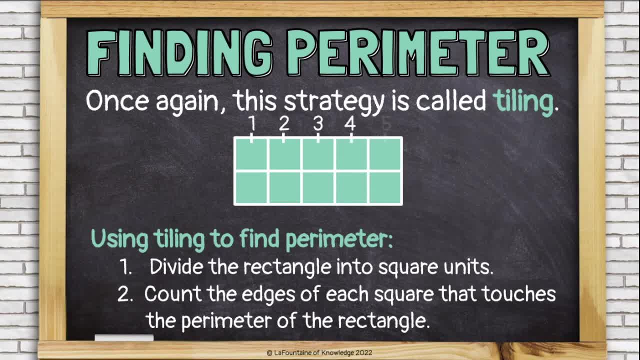 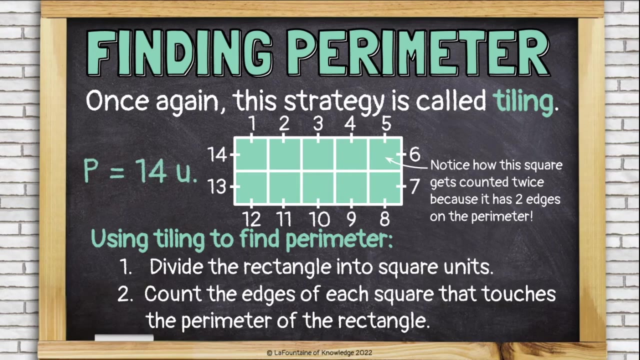 two, three, four and a half, 4,, 5,, 6.. Notice how this square actually gets counted twice, and that's because it has two edges on the perimeter: 7,, 8,, 9,, 10,, 11,, 12,, 13,, 14.. This has a perimeter of 14 units. 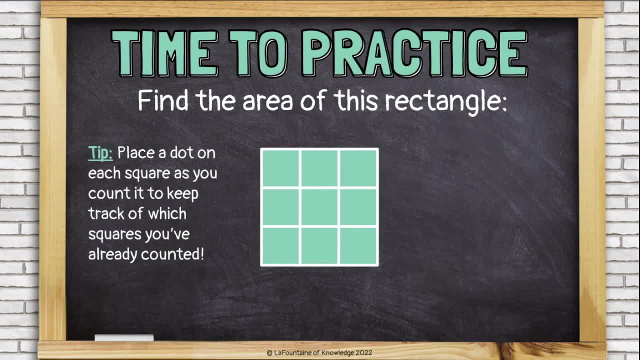 Let's try one more area problem. When you're doing this on paper, a good tip is to place a dot on each square as you count it, to keep track of which squares you've already counted like this: 1, 2, 3, 4, 5, 6, 7,, 8, 9.. This shape has an area of 9 square units, Remember. 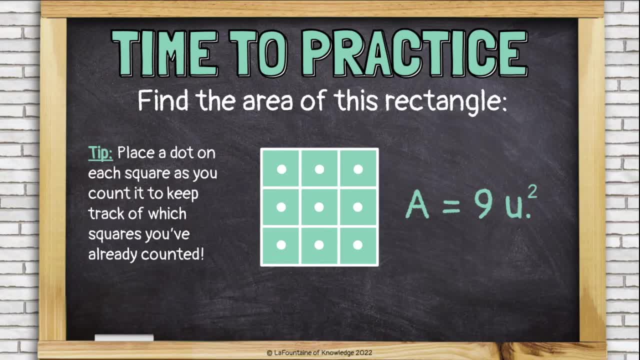 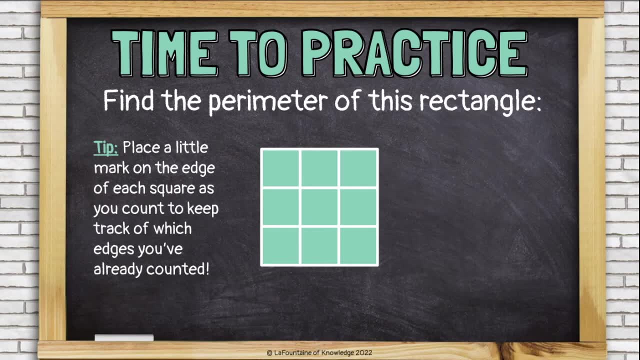 area is how much space fills the inside of the shape. so if we simply count how many squares fit inside this rectangle, we have found the area. Practice one more with perimeter, and my tip for perimeter is to place a little mark on the edge of each square as you count it, to keep track. like this: 1, 2, 3,, 4,, 5, 6,.